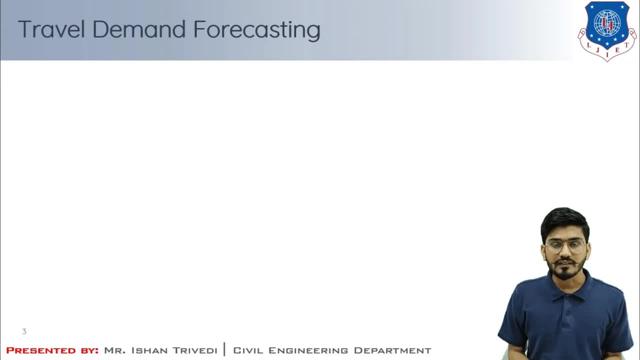 population and land use pattern of the city area. I will further discuss these things and the calibration of forecasting techniques. Then, third, is the forecasting of future and conditions, And at last is an analysis of future transportation systems, which also provides for the essential feedback between the transportation and land use elements. The inventory provides the base upon 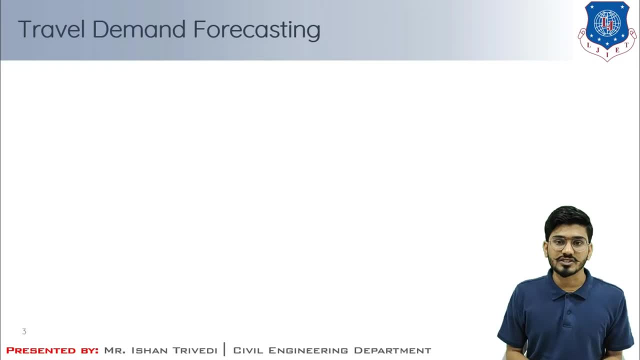 which the transportation planning process rest, and these includes surveying of economic surveys or activities, then population, as I said, then measure of land use and the distribution of land use and particular city area and basic travel characteristics of existing transportation facilities. Then in the analysis part, or I can say in analysis and calibration phase, the data resources of the 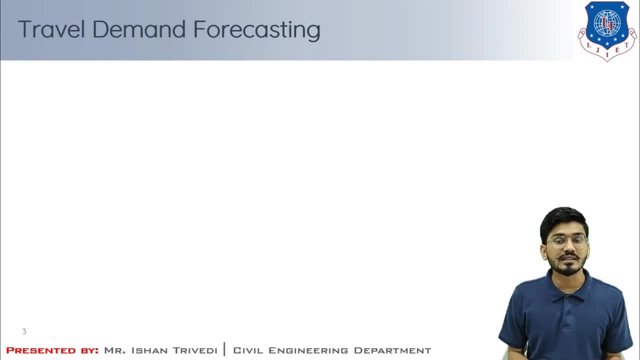 inventory phase are analyzed that we have captured in the inventory phase and then the forecasting techniques are used for the further development. Here the primary forecast are the estimation of the future population. First we need to calculate the future population based on the past trend or 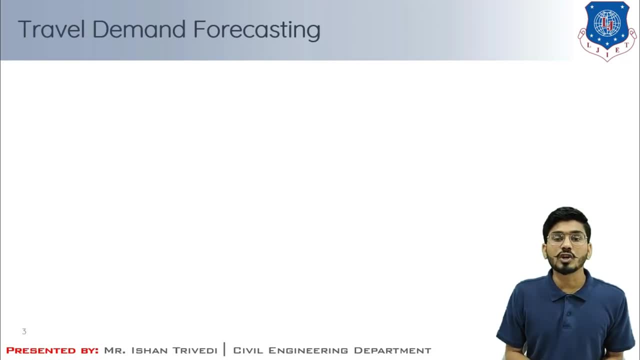 the past decadal growth and then the level of economic activity, usually expressed in terms of employment or the income, and these will be studied in the study area. Land use phase. translates the population and employment which has increases into land requirement and allocate them to the individual. 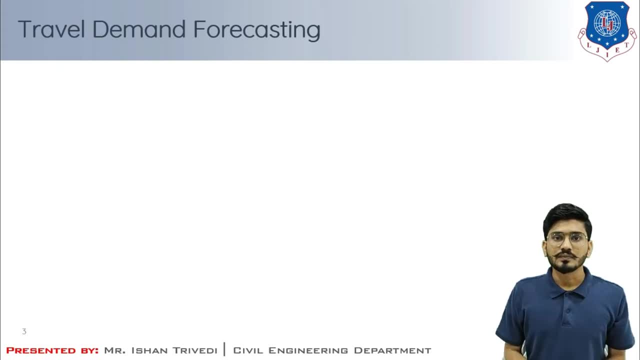 analysis of various units. Now, trip generation, bridge the gap between the land use and the travel by providing the means with which the number of trips that has begun, or you can say end, in a given analysis unit which can be related to the land use, socio-economic characteristics of that particular. 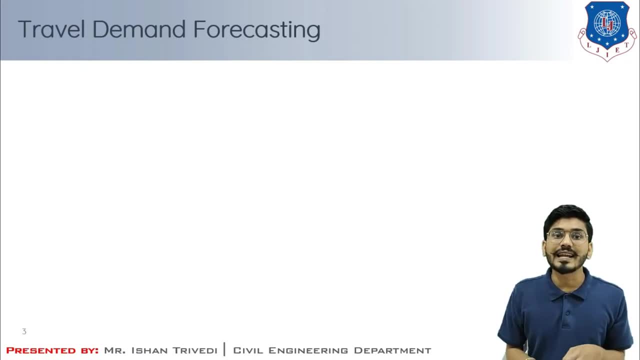 unit. So whatever the trip has been generated that is related to our land use and socio-economic activity- Remember those things we are going to talk about in the next part of this video, So this will come up in just next few minutes. So what? whatever has been generated in trip generation. 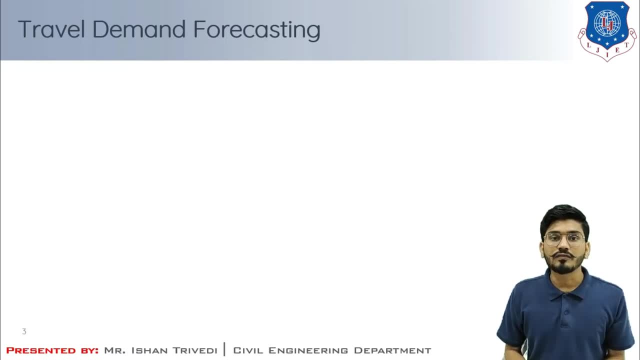 those trip ends are of land use and of those socio-economic activities, Then these generated trips ends form the measure of trip production and attraction, which is part of trip generation. or you can say the origin part and the destination. Later you will understand these terms as well Then that 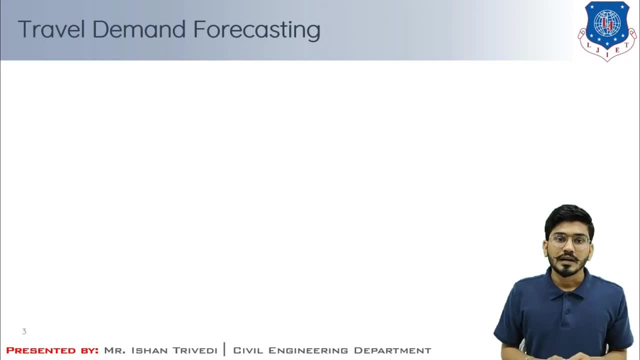 will be used in the trip distribution. After that those measures has been taken in the spatial form and the area wise, and the development from highway and transit network is being estimated with various travel patterns. These travel patterns are then assigned to the highway or transit network in the traffic assignment element In the transportation system analysis phase. 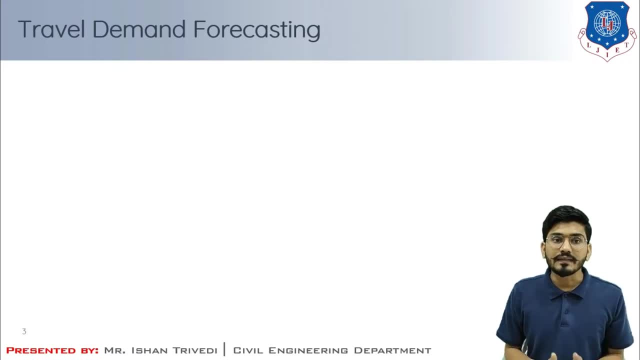 any alternative of both land use plan and the transportation system can be evaluated. The objective of transportation planning process is to provide the information necessary for the making the decision on whom and when and where the improvement should be made in the transportation system and thus satisfying the travel demands and promoting 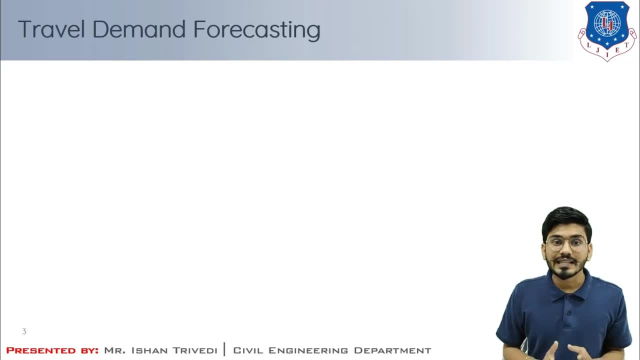 the land development pattern that are in keeping with the community goal and the objective. So there are clear picture of the these logical sequence of this technical element, and there has been certain question has been raised in your mind as well. For example, the population and economic studies has been done in the inventory. then what will be? 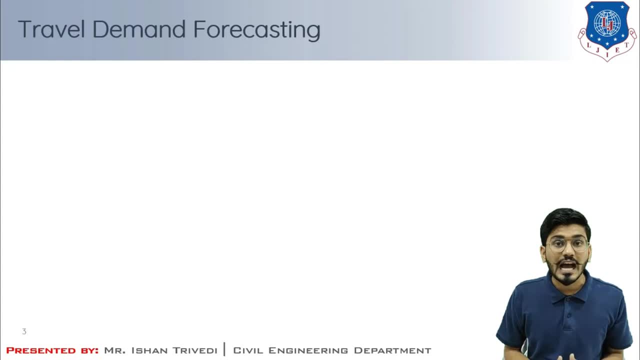 the magnitude of these activities, What is the amount of those activity and how these activity has been distributed. Then, second is land use. where will activity are been located Then? just because of your house, to college house, to workplace, what you have, the activity has been. 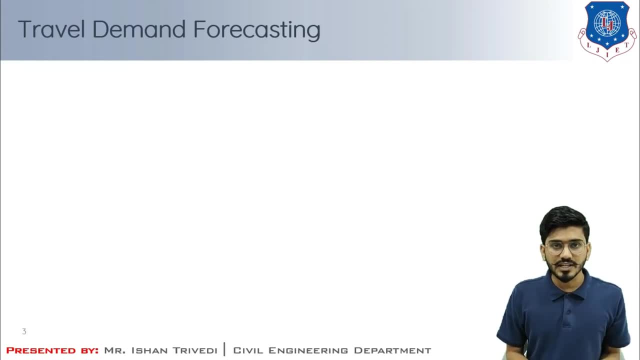 distributed just because of land use, Then trip generation means: how many trips will these activity generate? So now, based on this concept, I will discuss about the four steps of travel demand forecasting models. Here, this transportation forecasting is the process of estimating the number of trip that 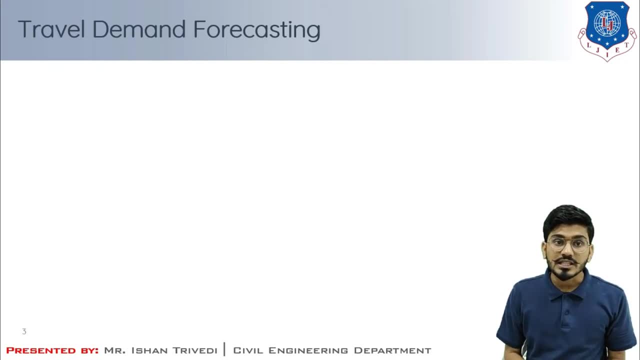 people will use a specific transportation facility in the future. For instance, a forecast may estimate the number of trips on a planned road or bridge Here, the ridership on the bus services and the number of passengers which are visiting at the railway station, bus stops or. 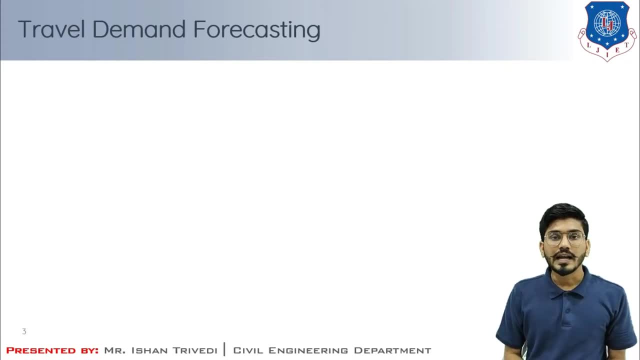 any airport. So what I will do, I will make a forecast of those transport facilities and those ridership of the bus service or the railway station or any airport. I will make those studies on those ridership and again, the forecasting of those trips will be estimated. 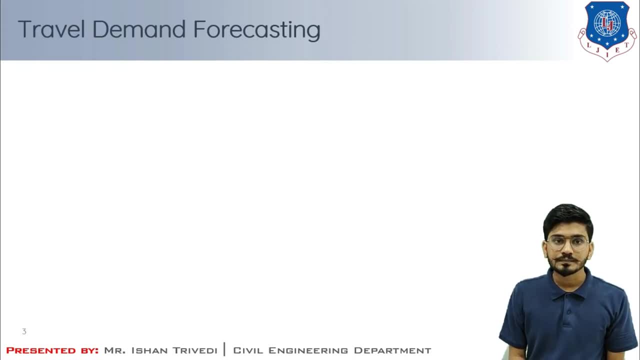 Here, this traffic forecasting begins with the collection of current traffic data, and this traffic forecasting is done with the help of direct traffic data, And these traffic data is combining those data and the other known data as well, such as population, employment, trip rates, travel costs and so on, to develop a travel demand model for the current situation. 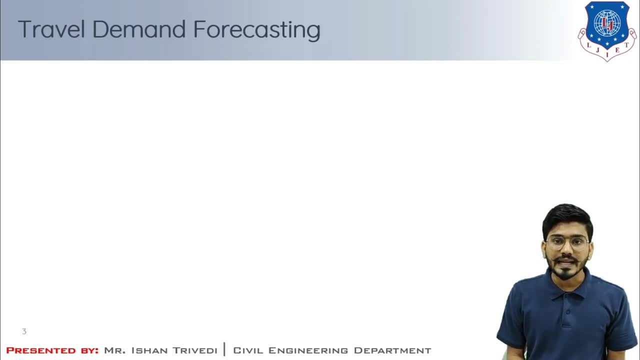 Feeding it with the predicted data for the population, or you can say employment, which results in the estimation of future traffic, typically estimated for each segment of transportation infrastructure in question, For example, roadway segment. or you can say railway station or any traffic management. 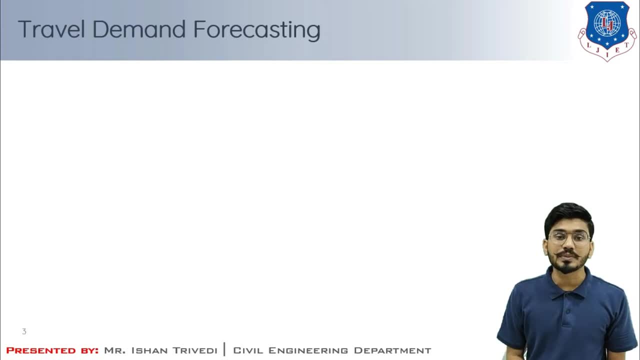 Here the traffic forecasts are used for several key purposes in the transportation policies Planning and management and the engineering to calculate the capacity of the infrastructure, For example bridges. where do we locate the bridges? how those bridge design? is there then road capacity? or you can say road width? 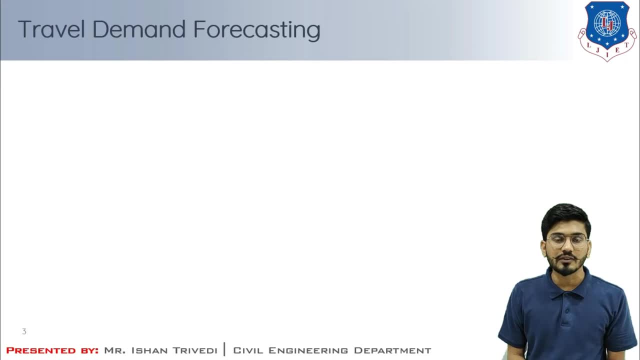 If you want to extend the road width, you need to calculate- and you should have those forecasting- How much will be the traffic in the future. If any places are there for the junction, particularly where we require over bridges, then we can calculate the traffic in the future. 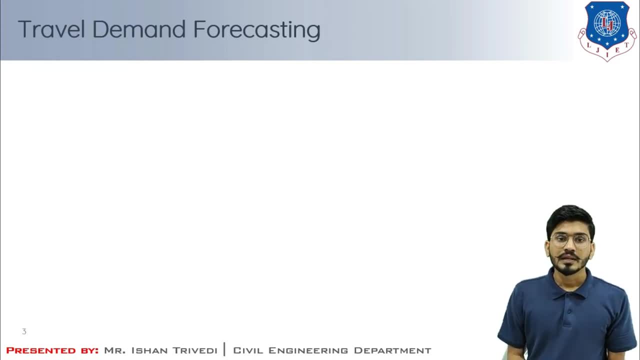 If any places are there for the junction, particularly where we require over bridges, then we can calculate the traffic in the future. These are some of those examples. Then the financial, economical and social viability of the infrastructure project, using cost-benefit analysis and social impact analysis and environmental impact within the rational planning framework, and the transportation forecast have traditionally forwarded the sequential step, or you can say sequential four steps, of the model. 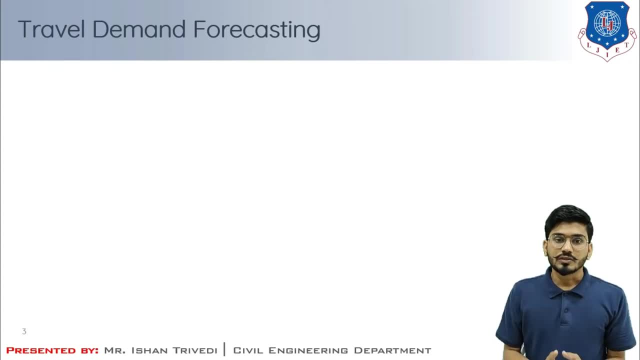 Or you can say urban transportation planning process, So transportation forecasts are made for the region as a whole, For example a population growth and its land use. Then this region is divided into zones and by trend, or you can say regression analysis, and the population and the employment are determined for each zone, and thus this calculation has been done. 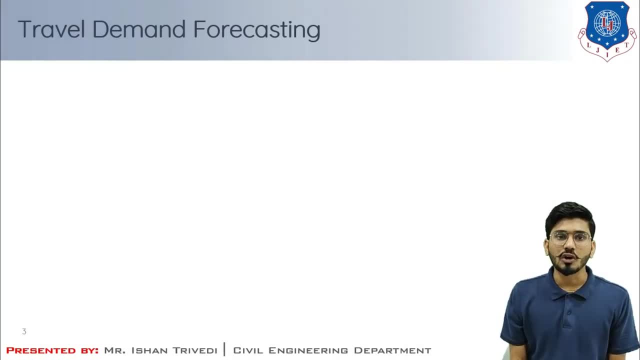 So the four steps of classical urban transportation planning system model are dependent on the land use characteristics. As I said, these are of socio economic activities and these ultimately generate the trip generation, or you can say here the zonal trip, and calculation has been made. 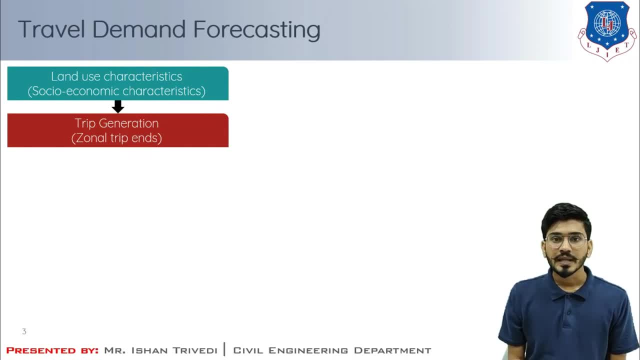 This determines the trip generated from each zone by trip purpose. This determines the trip generated from each zone by trip purpose. This determines the trip generated from each zone by trip purpose as a function of land use and household, demographic and other socio-economic factors. for origin: 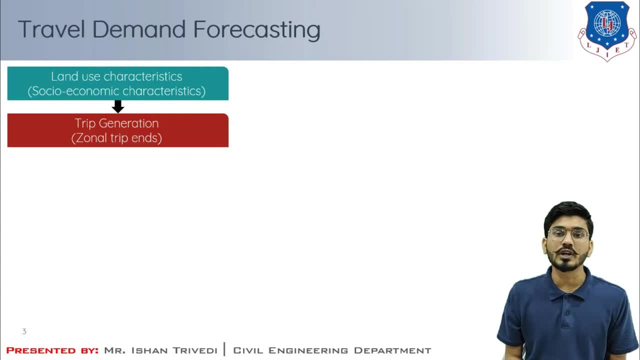 or destination and, as I said here, the calculation of zone trip end will be done. Then, after trip generation, there is a trip distribution which matches the origin with the destination and often using a various growth factor methods, or you can say gravity model function which are equivalent to an entropy maximizing. and here the trip interchanges. 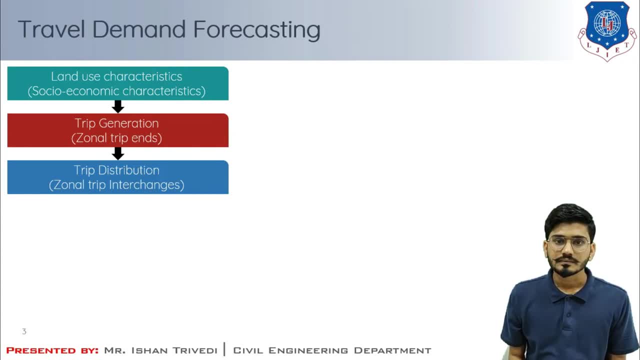 are done. Then there is a mode choice, or you can say model split. Mode choice computes the proportion of trips between each origin and destination and that use a particular transportation mode use and logit model to find the mode use and destination used by the trips, and here the sharing of various trips will be calculated. 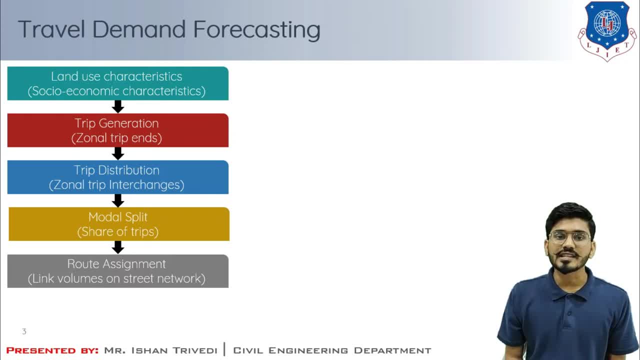 And, at last, route assignment. Route assignment allocates the trips between an origin and destination on particular. Often word draw principle of user equilibrium is used where each person or trip use the shortest path. subjected to all the person or trip doing the same, We generally adopt shortest path and that is what in route assignment has been done. 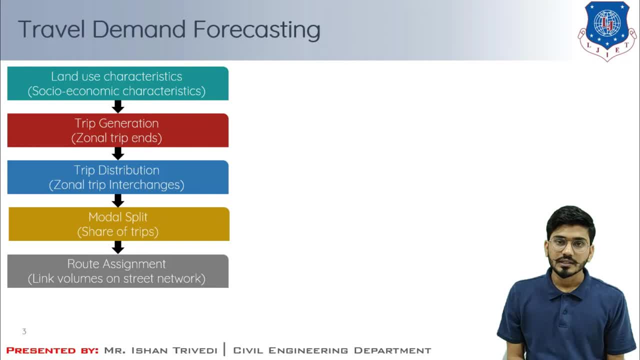 And here the transit network or street network will be studied. The difficulty is that the travel time are a function of demand, and while this demand is a function of travel time, and so we call it a bi-level problem. Now understand this by an illustration. 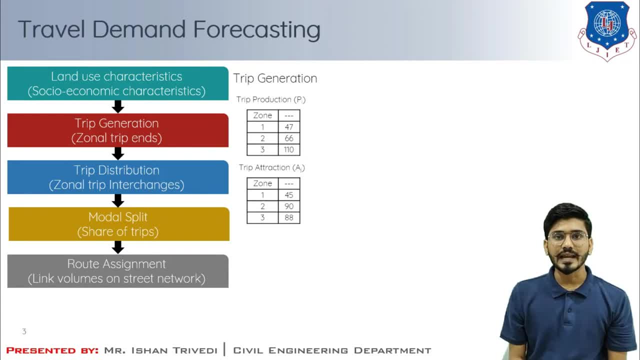 As I said, In trip generation there is an origin and destination. Origin belongs to the trip production from various zone those trip has been produced and which has attracted towards another zone. For example, you are living in your zone area where your house is there and you are going. 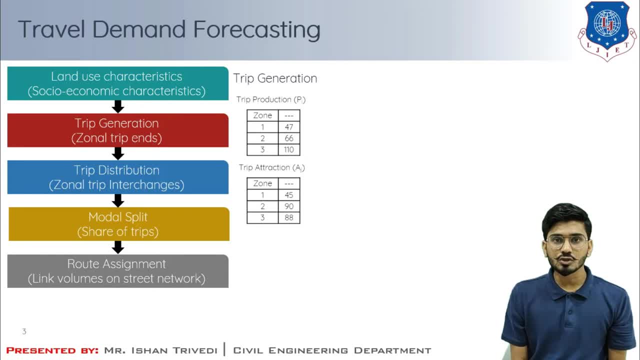 towards a college which is at located at different zone, Then your trip has started. or begin with the origin and that is your trip production. Your home is trip production and your destination or your end trip is the trip attraction. Here you can see in trip production number of trips has been shown. 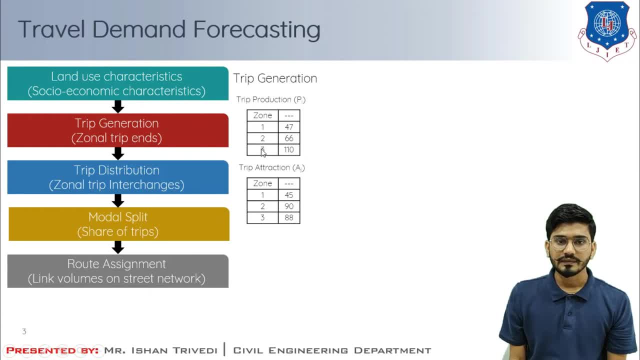 Here you can see, in zone 1 there is 47 trips, then in zone 2 there is 66 and in 3 it is 110.. These are generated, so it is a trip production which is denoted by pi, Then in attraction it is denoted by aj, and those are of 45.. 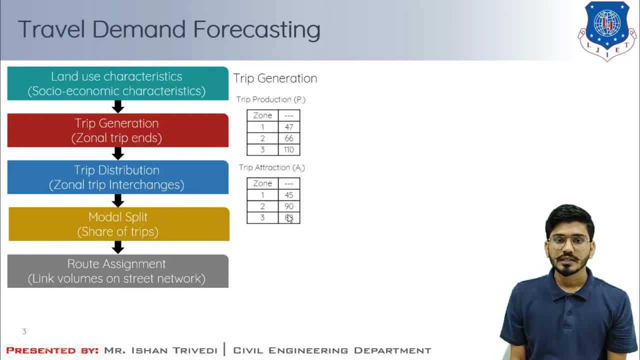 Then 90 trips going towards zone 2 and 88 are ending with zone 3.. So, among of all these, as we get this distribution of various interzonal activities, Now what I will do, I will do the trip distribution here. a matrix will be formed from which zone. 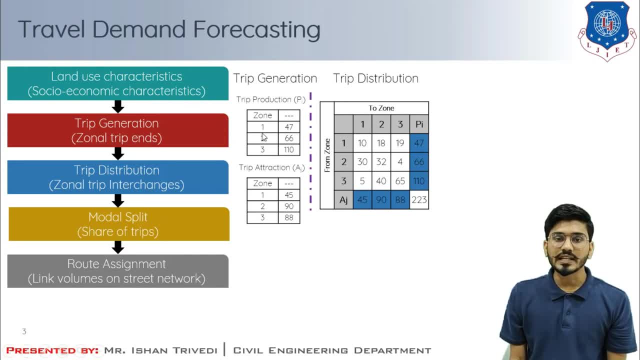 to other zone. So out of this, 47 activities which has been produced from zone 1. Which has distributed here, So within the one zone- here you can see 1 to 1 zone activity is 10.. From one zone to second zone there is an activity of trips of 80 in numbers. 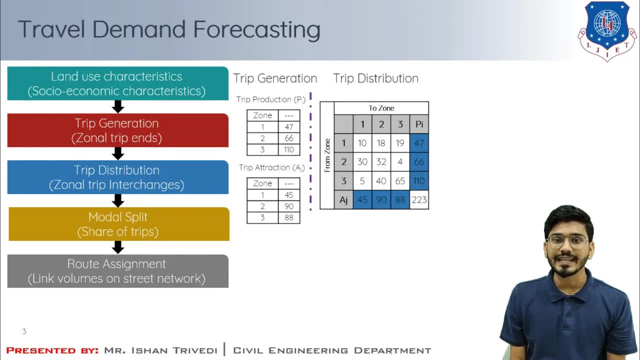 Then in from zone 1 to 3. it is of 19 in numbers. So this is how your activity has been distributed and if you make the summation, it will be same as those of trip produce From the zone 1. similarly, I have given the bifurcation of activities of these zone from: 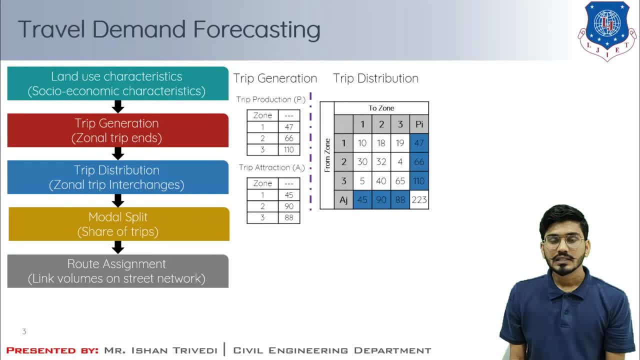 their origin to those zones as well. So here you will see a matrix form. it is of n by n matrix. the number of zone multiply with those destination number of zone. So it is of n by n matrix. you can say: and it is of n square. 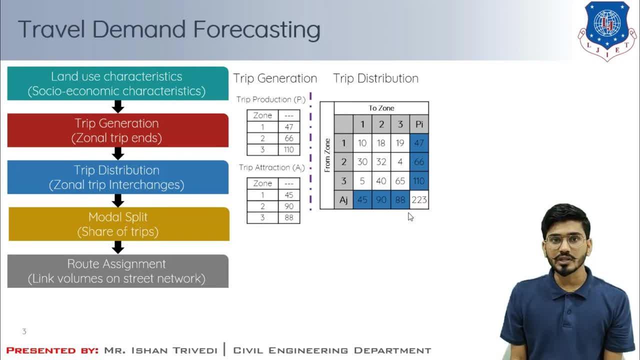 So these zone Are 3 in number, so here the matrix is 3 by 3.. This concept you will further understand in next lectures. So this is how these interzonal activities are distributed in trip distribution. So if I take example of this trip distribution, that from zone 3 to zone 2 there is a trips, 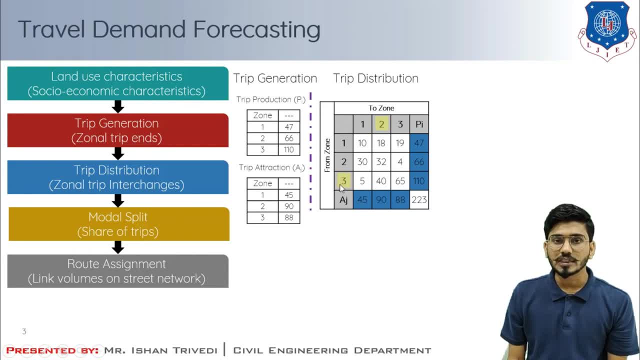 and these number of trips are of 14 numbers. so from zone 3 to zone 2 there are 14 number of trips. So this is how the model has generated and this bifurcation is also further goes to the model split Out of these 40 trips. how many modes are there which people have adopted to travel between? 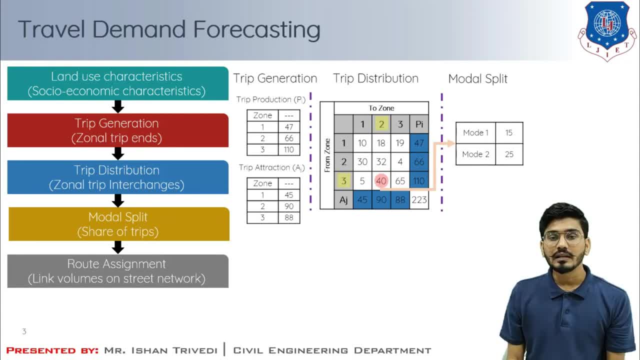 zone 3 to zone 2 and these activities are done in the model split and here the distribution of various modes. here I have taken just two modes. you can take others as well. How much detail, depth or factors you want to calculate, This has been studied here. 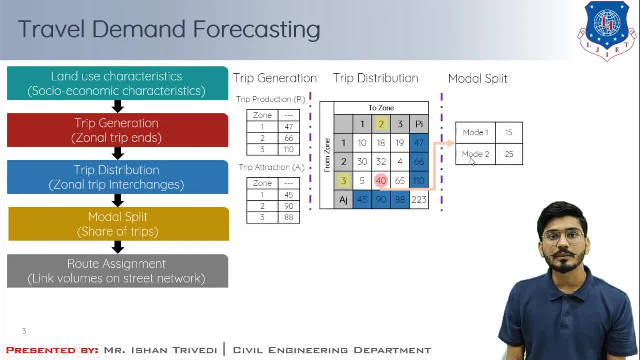 So here mode 1, for example cars, and mode 2 is the public transport. 15 number of people have travelled from zone 3 to zone 2 by car and for public transport it is of 25 trips. From this model. split out of these 25 trips how they have assigned their routes there. 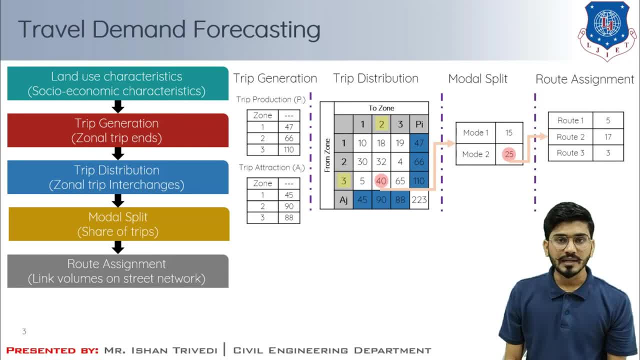 are ample of routes, So again there is a route assignment. There are ample of routes, So again there is a route assignment. They have gone from zone 3 to zone 2, that is okay, but which route they have opt? Here again, the detailed study of route classification is made then, and that is what our travel demand. 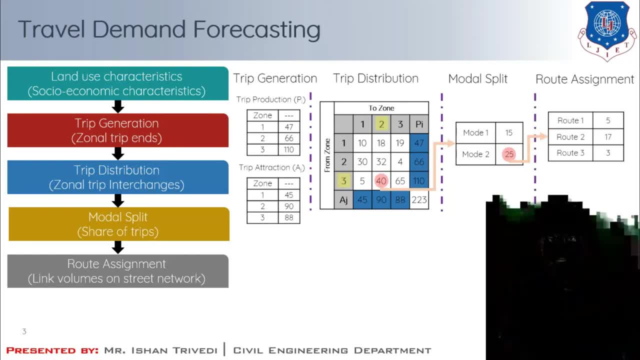 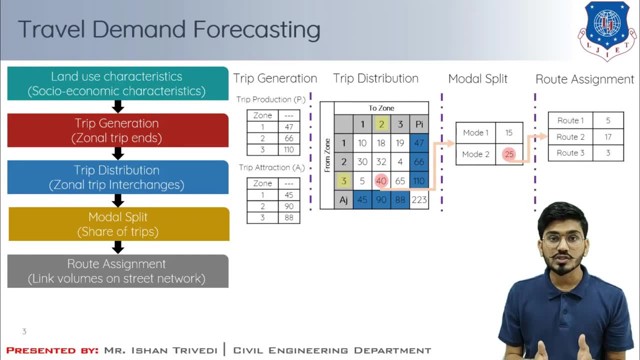 forecasting. and these four steps illustrate this generation to route assignment. So how they have, opt the various routes and this is we are going to study their examples in the next upcoming sessions. So these are the basic concept of this travel demand forecasting And, you have to remember it, these are of trip generation. trip distribution model split. 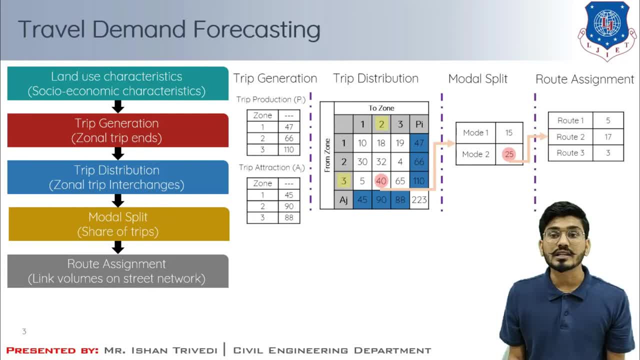 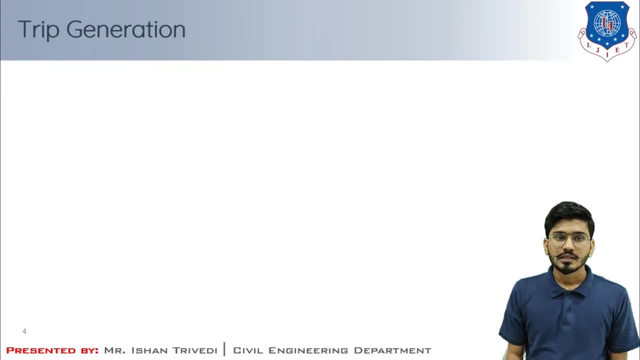 and route assignment. Route assignment sometimes called a traffic assignment. So first we will understand what is trip generation. The first phase of the transportation planning process deals with the surveys, then data collection and inventories, as I said Here. in next phase, The analysis of the data. 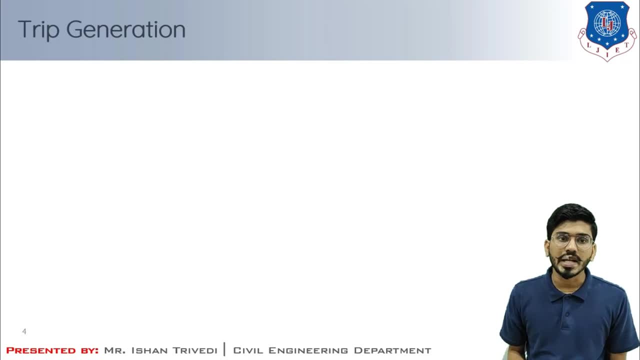 The analysis of the data. The data is so collected and the building model describe the mathematical relationship that can perceive in the trip making behavior, and that is what our objective. The analysis and the model building starts with the step that commonly known as a trip generation. 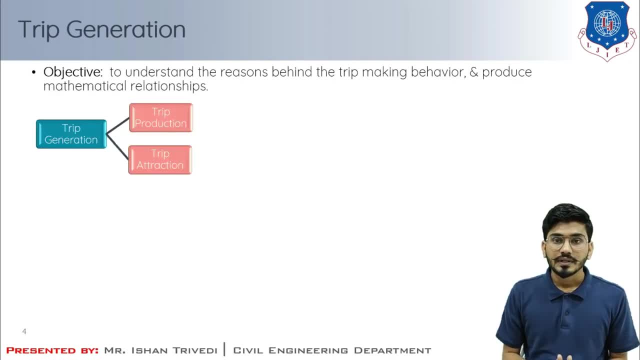 Here two types of trip generation analysis are carried out, and these are of trip production and trip attraction. If I am talking about trip production, then it reserved for the trip generated by the residential zone where the trips may be trip origin and destination. Then trip attraction is used to describe the trips generated by the activity at the non. 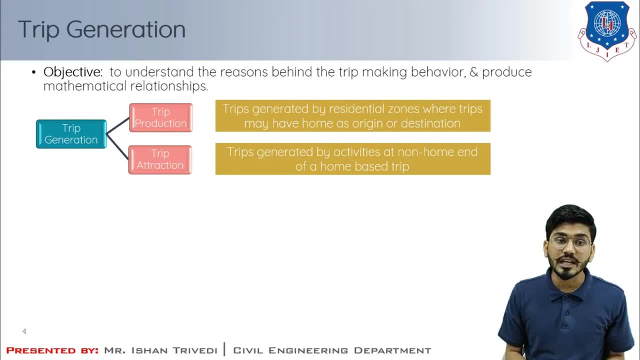 home end or you can say a home based trip, such as employment, retail service and so on. The trip generation is general term used in the transportation planning process to cover the field of the calculating the number of trip ends in a given area. These things already I have been taught you. 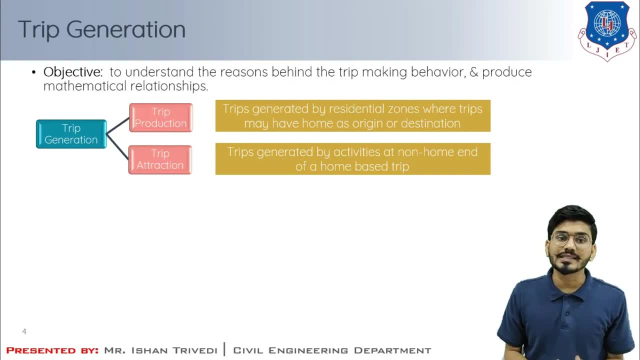 The objective of this trip generation stage is to understand the result behind the trip making behavior and to produce the mathematical relationship to synthesize the trip making pattern On the basis of observed trips. The trip generation is general term used in the transportation planning process to cover: 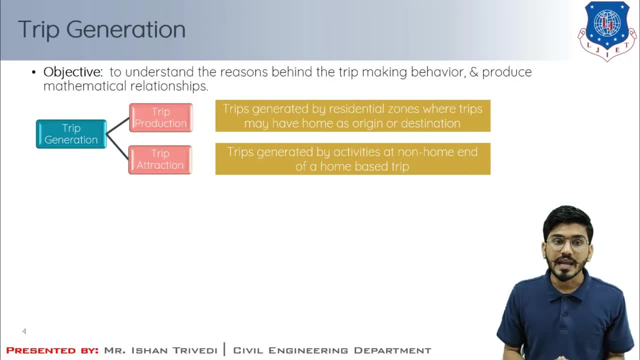 the field of the calculating the number of trip ends in a given area. The trip generation is general term used in the transportation planning process to cover the problem of the trip meet. the Judeiros range of simplest is not aquela area. The trip generation is general term used by meetings in non normal time. 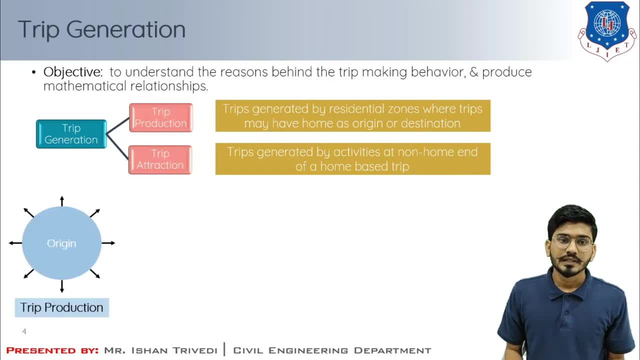 Here the rep tuvo idea, followed by troublesheet, Once again the trip generation test in COD. First of all, as temporary trip, there is발 two trip ends: one is trip production and another is trip attraction. means trip origin and the destination. These two trip ends, as I said, the origin, that is starting of the trip, and the destination. 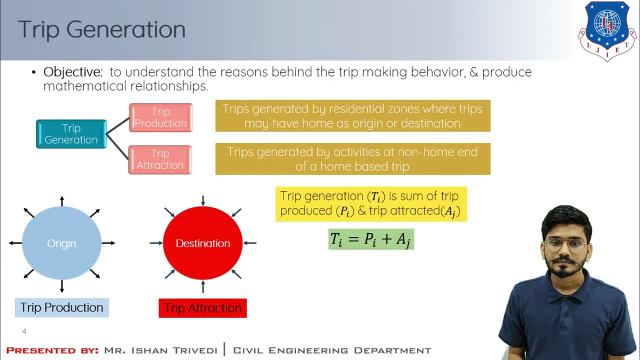 of the trip. So here, this trip generation, that is denoted by Ti. capital Ti is the sum of total trip produced, and that is Pi, and total trip attracted, that is Aj. So capital Ti is equal to Pi plus Aj. that you have to remember here, the total trip generation. 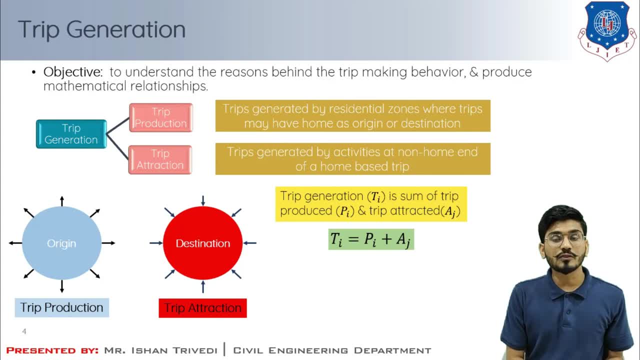 is summation of total trip produced, that has produced from the origin and it has attracted towards a destination and that is called the trip, and or you can say destination, and it is the summation of total production and total trip attracted. Furthermore, let us understand what is trip purpose. 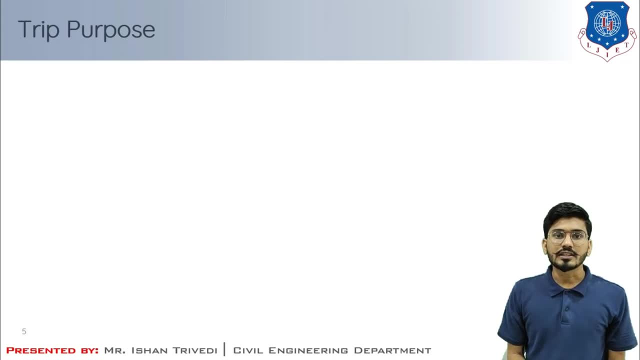 Trips are made for the different purposes, and thus classification of trip by purpose is necessary. If I am talking about important classes of those trip purpose, these includes of work trips, business trips, college or school trips, then social and recreational activities, and there are sports and other activities as well. 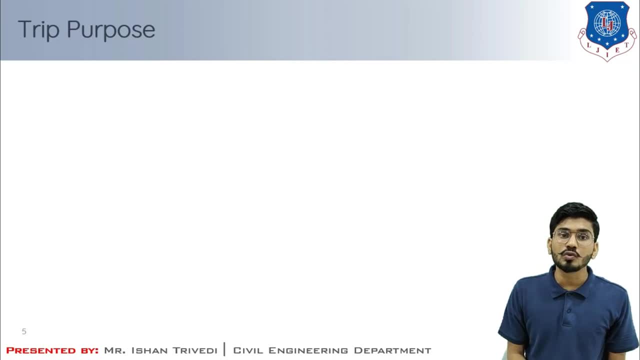 So the trips are usually divided into three categories. The trips are divided into three categories. The trips are divided into three categories. One is home based trip and another is non home based trip. If I am talking about the home based trips, then these are having one end. or you can say: 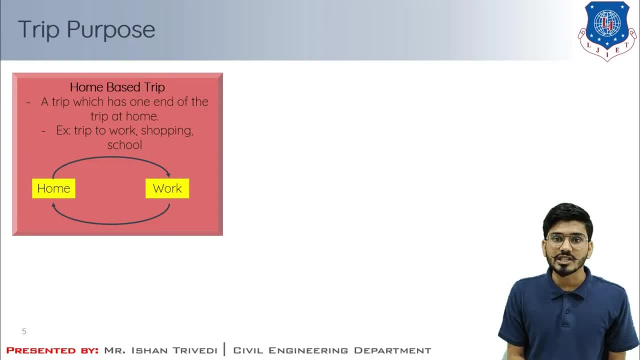 one end of the trip, either origin or the destination at home, and here the person who is making this trip, their any origin or end is home and while if I am talking about the non home based trip, these are having non home based trip. So this is the definition of having neither end the home of the person who are making 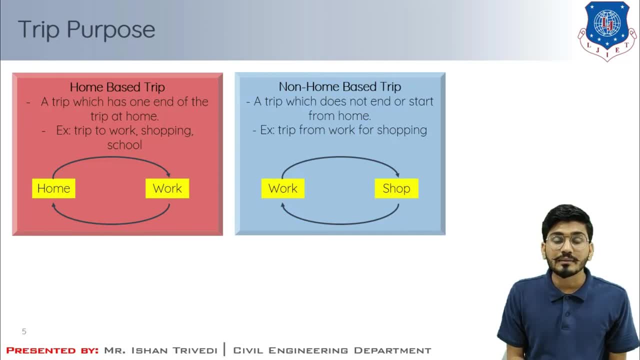 the trip. So this two definition are further classified by the few examples, as I shown you here. consider a trip from home to work and then return trip from work to home. both these trips are home based trip Because one end of those trips is home based trip. 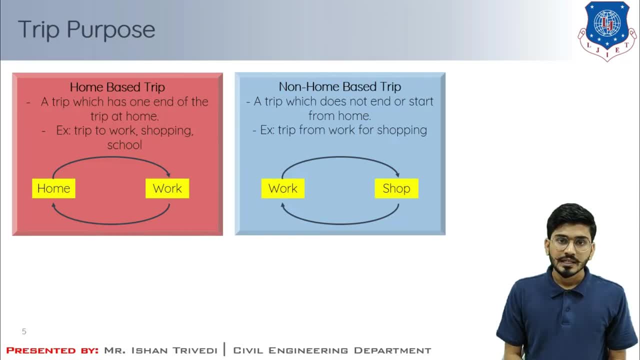 But how do we classify as home based trip? So what are the home based trips for us? Hmmm, home here, then both these trips are considered to have been generated at work zone and home have to to work to in number. home have to work purpose, which? 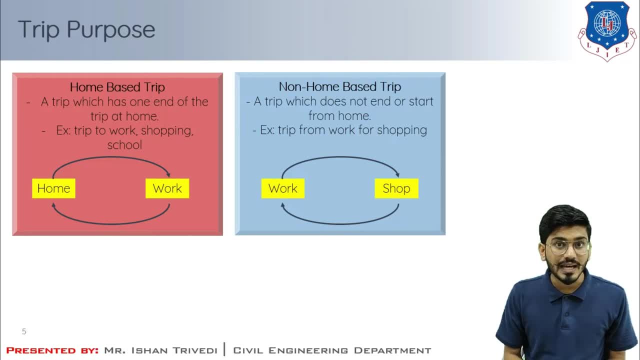 has attracted in the work zone. these trips are done at work zone, which has two in number home attraction, and that is of from the work zone. now consider another example of the trip from place of work to shop and return to the place of work, as it is usual duringPHD lunch time or 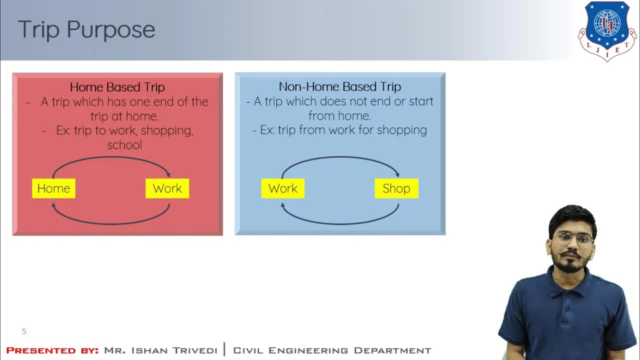 recess in most of the offices, then both the trips are of non home base trip, because neither end of megabays trip or house trip are of non home based trip. C, csak an example, is a non-home base trip. that is, of week day trip and of workspace trip and return of work times. the 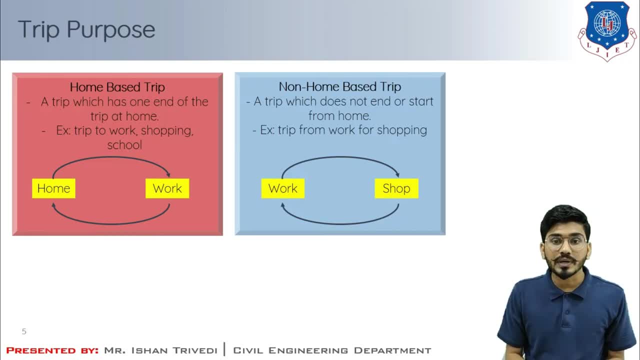 the trip is of home, of the person making the trip. here, both these trips are considered to have generated at work zone and attracted towards shop. earlier, what was that? the production from home and attracted towards work. now, here, the work zone attract these attracted towards shop zone. and now, if I am, 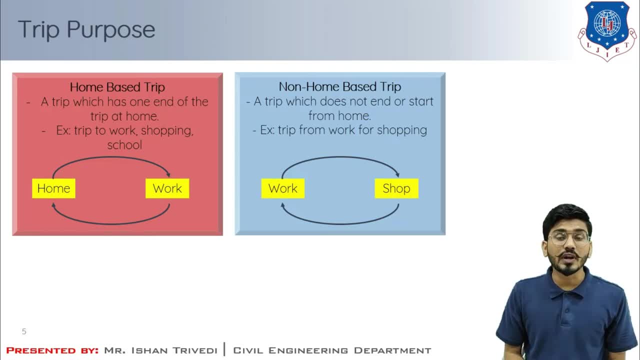 talking about the total summation, then it is four in number. one is home to work and work to shop, then shop to work and work to home. so total four number of trips has been generated. work is work zone and second is shopping zone. and this is how these about those definition and the concept that I have told you. 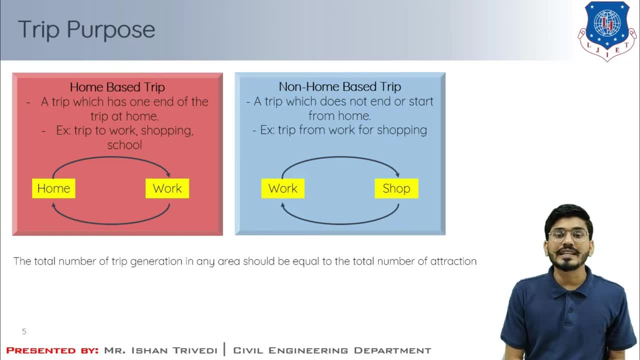 that the total number of trip generation in any study area should be equal to the total number of trips. attractions. here the breakup of those trip purpose is normally done for the home based trips, which represent almost eighty to ninety percentage of total trips, means the trips that in general form that happen. these are of home base trip in. 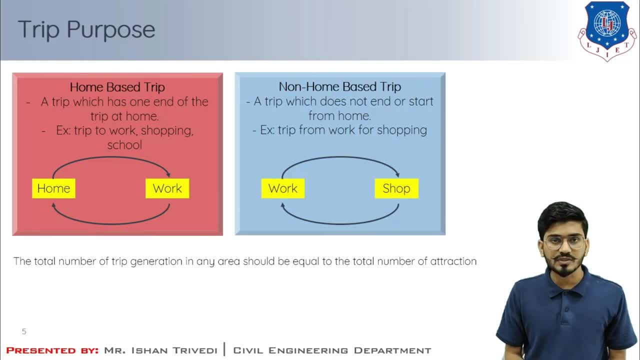 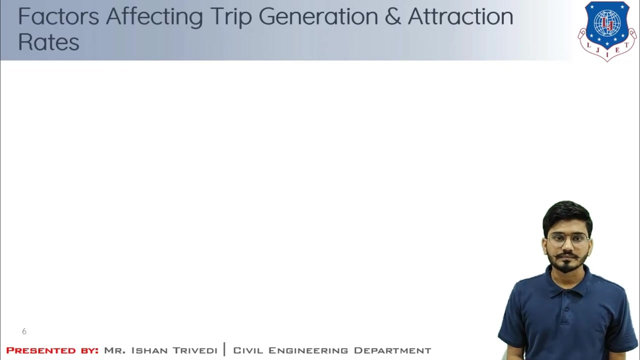 nature most of the time. only 10 to 20 percent trips are of no one home based trips. so these are the concept of trip purpose and divides the trips into two parts, that is, home based trip and non-home based trips. Now understand the factors affecting trip generation and attraction rates. 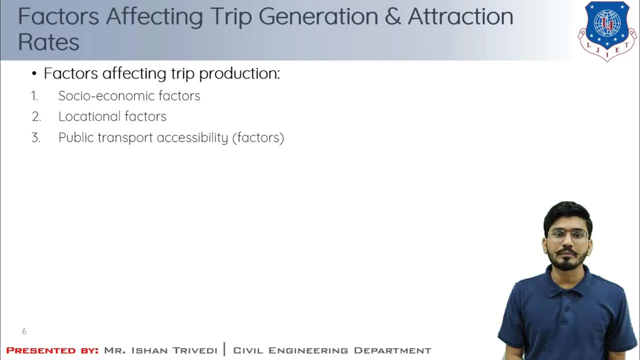 These are of socio-economic factor, location factor and public accessibility factors. If I am talking about the socio-economic factor, these are of household income, car ownership, family size and composition of household, or you can say household structure and occupational status. Then location factor includes the land use characteristics, residential, commercial. 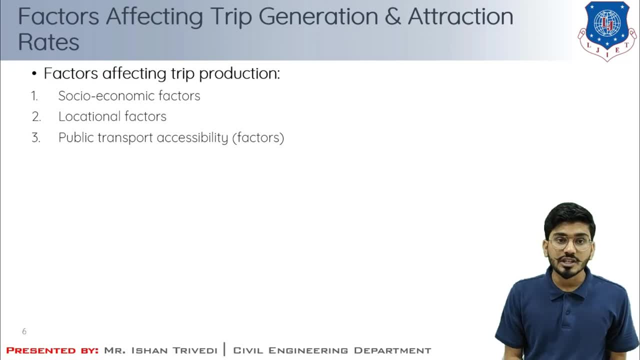 industrial, the distance of residential from CBD area, then population and the residential density as well. Then, if I am talking about the public transport accessibility factors, these include the accessibility to public transport system and its effectiveness, Nearness of public transport facilities, like location of bus stop or local train or local 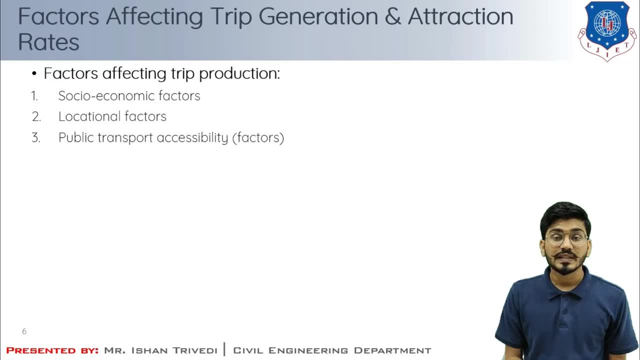 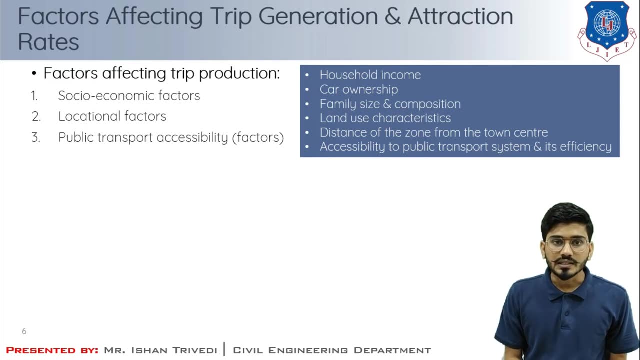 train stops, then their fare structures and routes. Here I am going to discuss few factors in detail. First is household income. Obviously, the family income will represent its ability to pay for the journey. These affects the number of trips which are generated by the household. 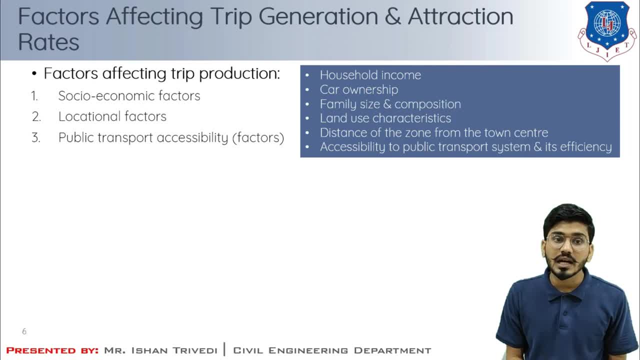 Here. higher the family income, higher will be the trip generation rate, So I will spend money on those trip generation. Then car ownership- usually a car owing household- will generate more trips than a non-car owing household. It has been said that by the same reasoning. 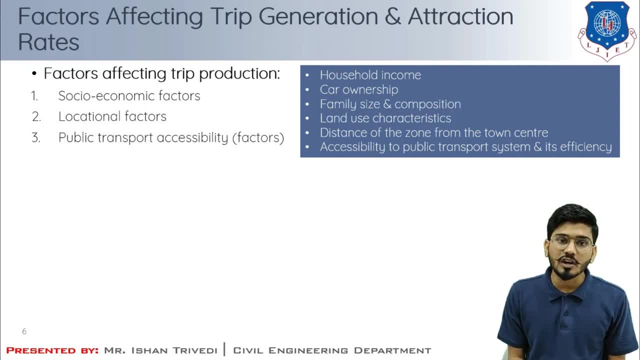 Like the way I have explained in the household income. the more number of cars in a household, then the more number of trips which are going to generate from that particular house. Then the family size and composition of household: The bigger the family, the more trips which are likely to be generated. 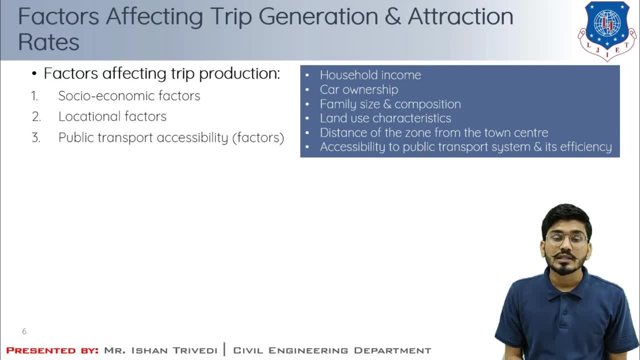 Further, it also affects both the nature or the structure of family as well. Further, if I classify That if the both person, like male and female, those who are employed or engaged in the work, then these trips generated will be more than when only one fellow is earning. 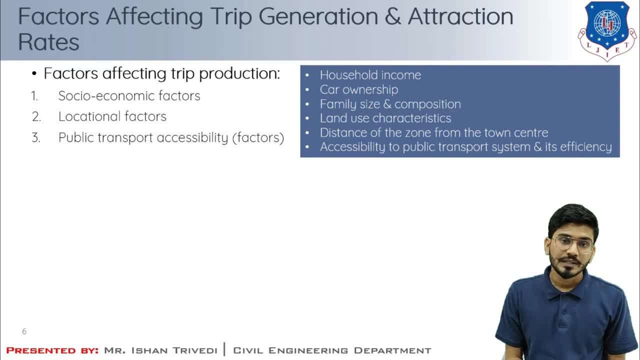 So employment also affects in this category as well. Further, if there are many school going children are there in the family, then the number of school purpose trips will be large, Then the aid structure will be larger, Then the family size and composition of household. 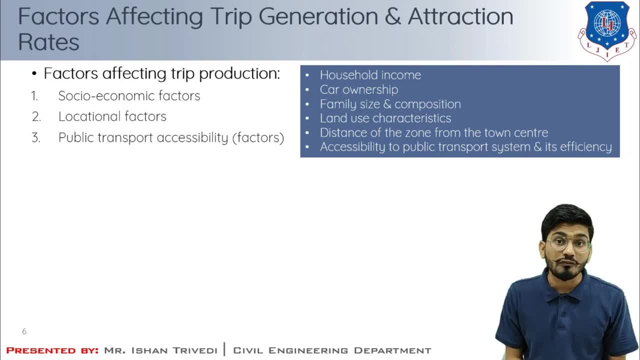 Then the family size and composition of household. So, as I said earlier, the structure of the household also affects here and the family. who are of more number in old age, then they are not going to generate any trips. So those who are old in age the old person, are not expected to generate as many as trips. 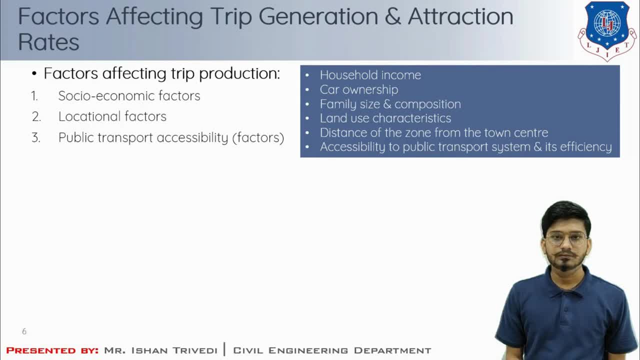 those are of younger one does. Then there is a land use characteristics. Different land use produce different trip rates. For example, residential area deals with the higher density of dwellings, which can produce more trips than the one with a low density area. 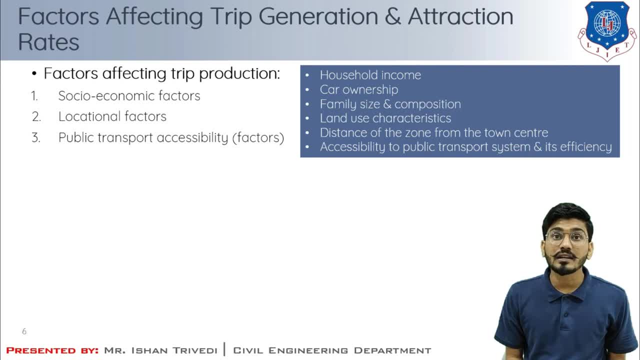 On the other hand, the low density area may represent luxurious bungalows which may produce a large number of private car trips. here the distribution or the various modes of transportation has been done And bifurcated. here. then the distance of zone from town center or the CBD area. then 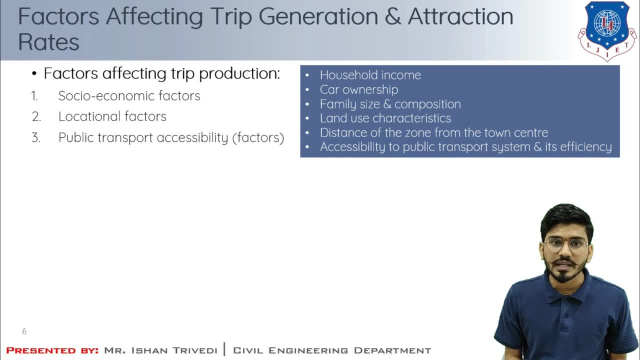 the distance of zone from the town center is an important determination of number of trips that people may likely to make to the town center. Obviously, the further the town center, the less number of trips which are likely to be generated in that CBD area. then accessibility to produce the public transport system and 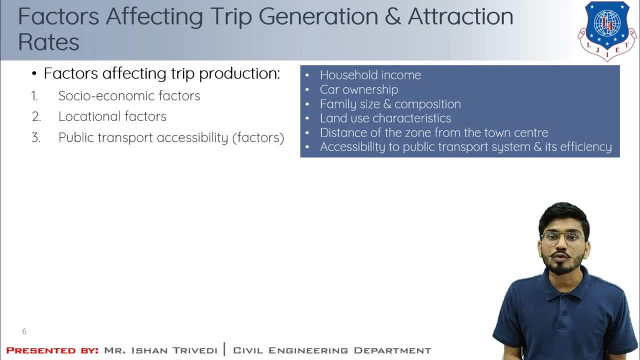 efficiency Here. easy accessibility to public transport system increases the desire of person to make those trips and generate more trips. See, in most of the sustainable cities or those who are of developed town, those who have well public transport connectivity, they have more number of trips. 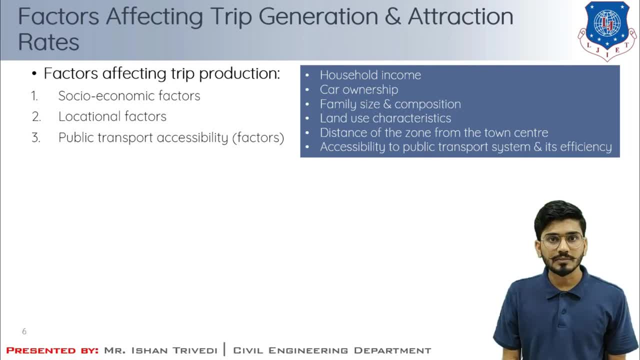 If I'm taking the example of Mumbai, Hong Kong, London public transport system than the Hong Kong, Many of those cities have more ridership because they have the connectivity from route level to the major modes of transportation. Now, if I'm talking about the trip attraction, which depends upon the activity and its concentration, 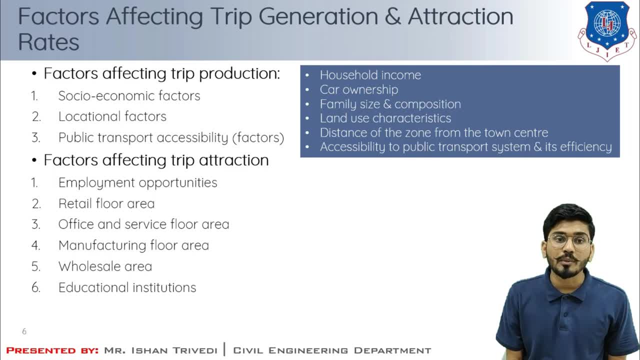 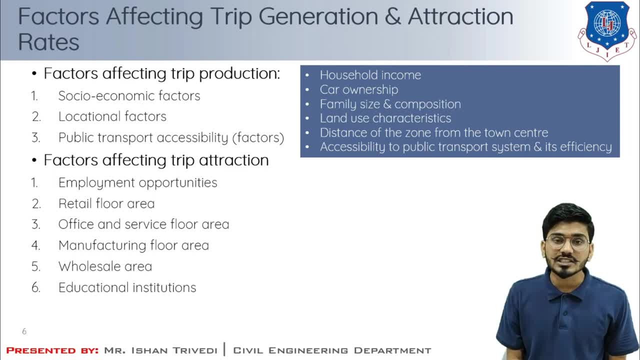 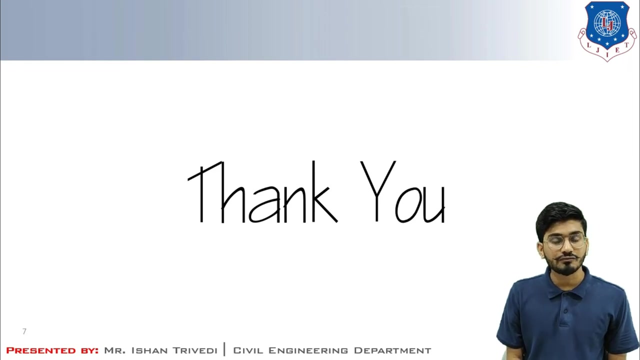 etc. The employment opportunities: often industrial or shopping units or you can say office establishment which directly governs the trip attraction rates. So these are the factors affecting the trip production and attraction rates. I'm ending this session here. I hope you have learned the concept of travel demand forecasting and first tip, that is of